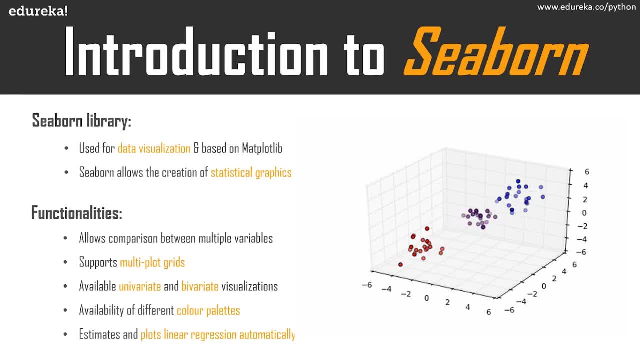 between multiple variables. It also supports multi-plot grids that, in turn, ease building complex visualizations. It has univariate as well as bivariate visualizations available to compare between subsets of data. the availability of different color palettes to reveal various kinds of patterns. 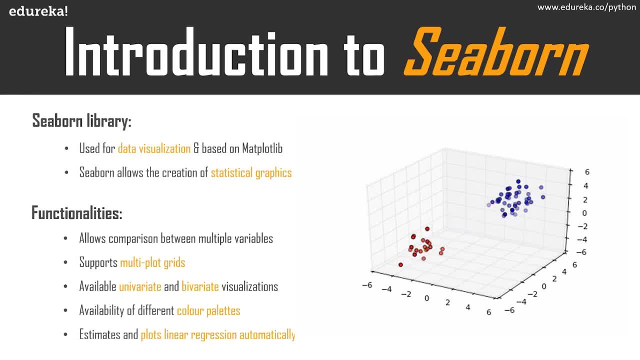 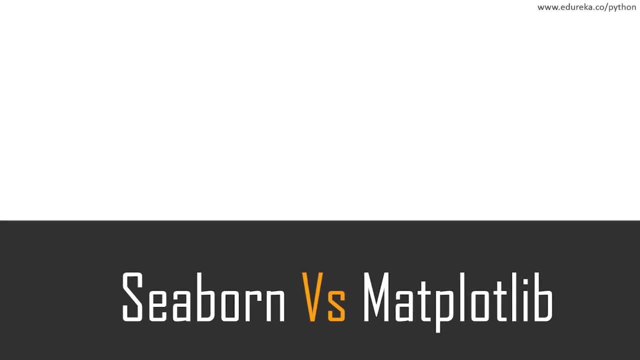 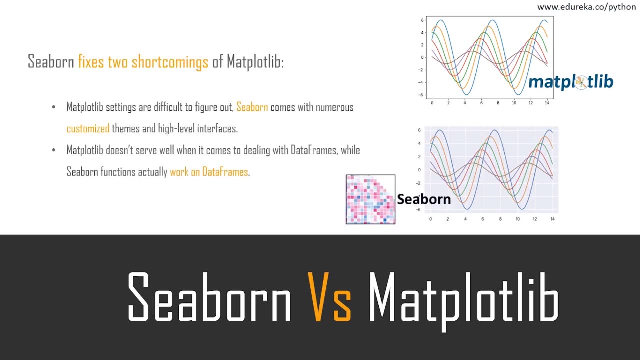 It also estimates and plots linear regression automatically. So now, if you were wondering why you seaborn when you already have matplotlib, here is the answer to it. Michael Vascom, who's the creator of seaborn, says: if matplotlib tries to make easy things easy and hard things possible, seaborn tries to make a well. 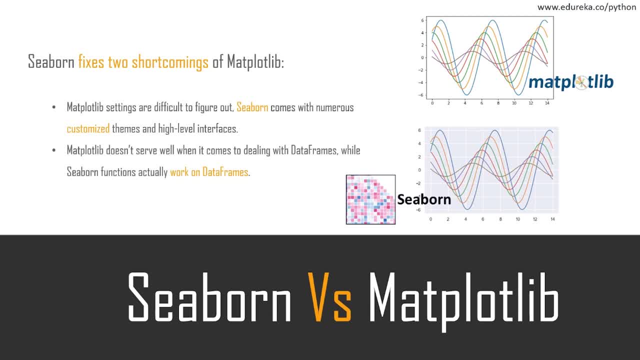 defined set of hard things easy to factually. matplotlib is good, but seaborn is better. There are basically two shortcomings of matplotlib that seaborn fixes. matplotlib can be personalized, but it's difficult to figure out what settings are required to make plots more attractive. on the other hand, seaborn comes. 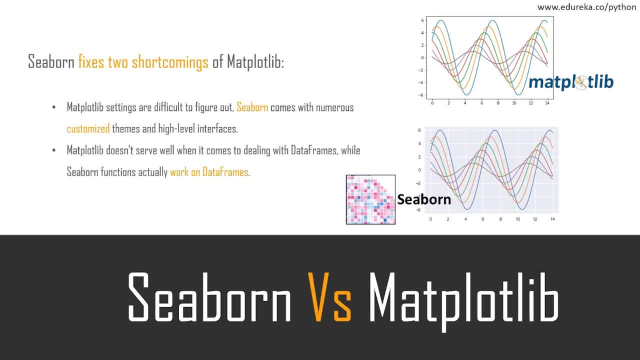 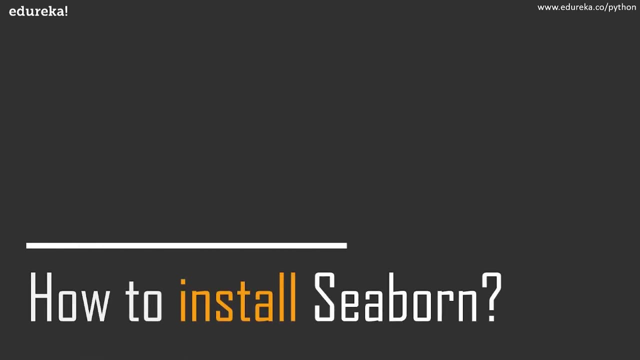 with numerous customized themes and high-level interfaces to solve this issue. when working with pandas, matplotlib doesn't serve well when it comes to dealing with data frames, While seaborn functions actually work on data frames. Now that you have an idea about seaborn, Let's move on to see how you can actually install this library. 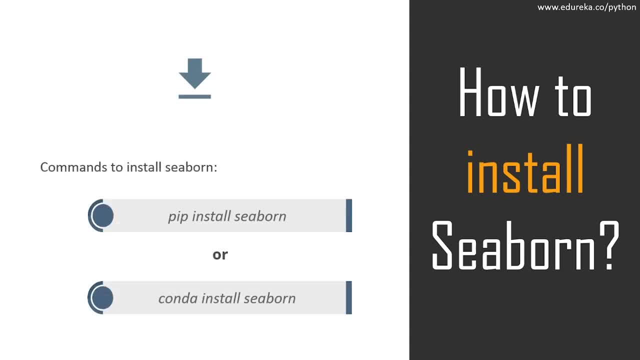 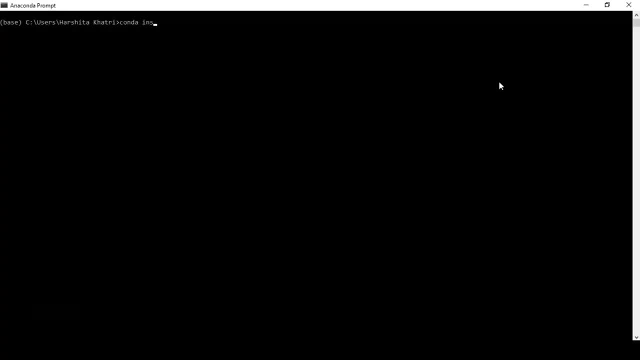 to install seaborn, You can use the simple pip install seaborn command or, if you are using an anaconda platform, you can just go to the anaconda prompt and type conda: install seaborn. Since I already have it installed over here, I'm not going to redo it again. 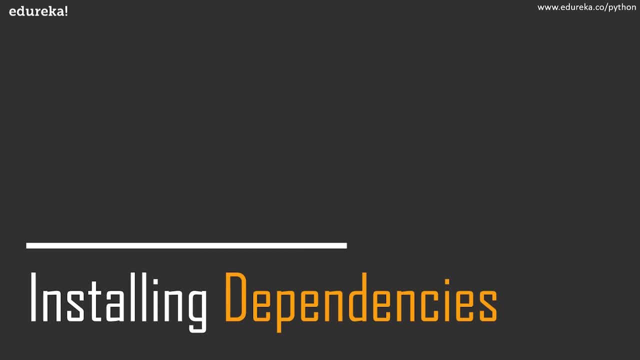 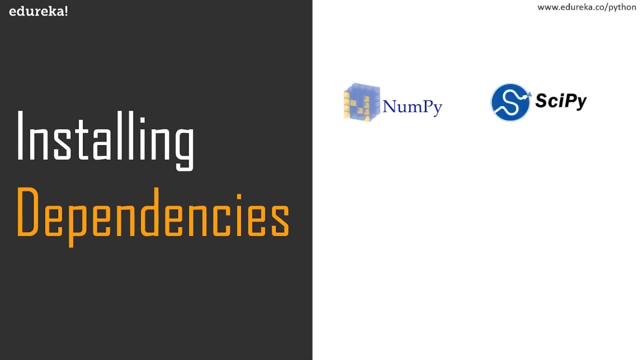 Now let's get back to our presentation and take a look at the dependencies of seaborn. seaborn basically has four mandatory dependencies, which is numpy, scipy, matplotlib and the pandas library. It also has a recommended dependency, which is the stats models library of python. 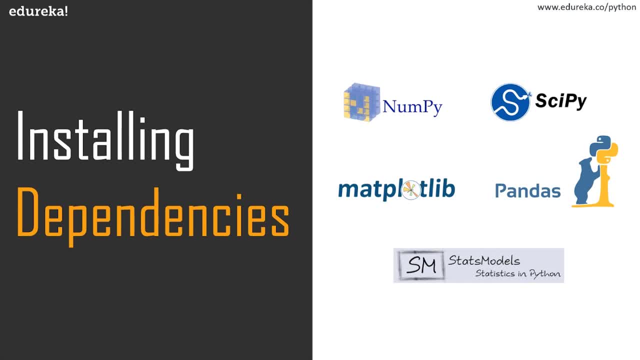 So, just like we've installed seaborn, We'll have to install numpy, scipy, matplotlib and the pandas library. to install these libraries You can use the same commands which I showed earlier with the name of go that particular library. Okay, so I hope everyone's clear till here. 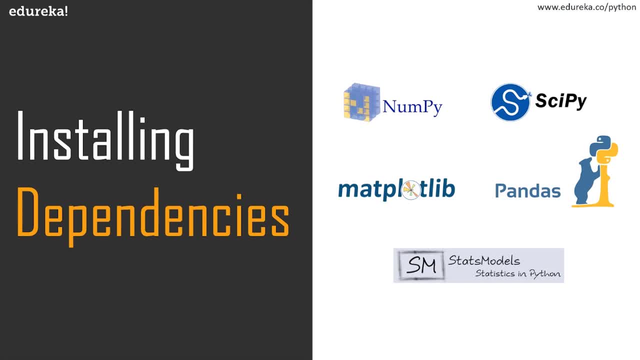 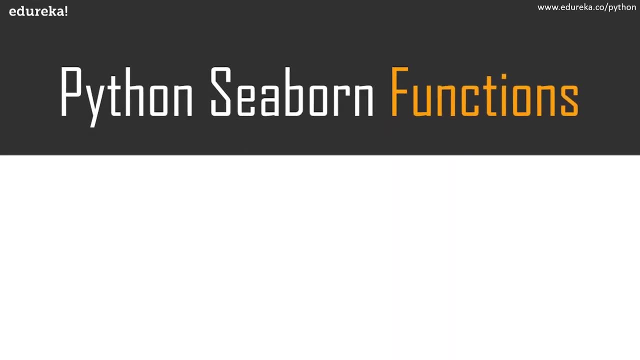 If you have any doubts, please do let me know in the chat box, and my team is here to help you. So now let's move on and take a look at the various plotting functions in seaborn. seaborn has a number of functions that are available for visualizing statistical relationships: plotting: 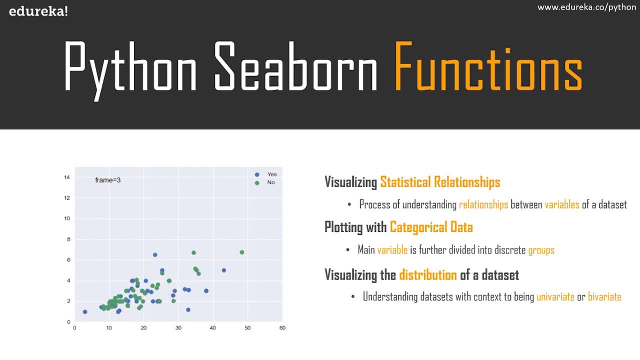 with categorical data visualizing the distribution of a data set. Let's begin with visualizing statistical relationships. the process of understanding relationships between variables of a data set and how these relationships in turn depend on other variables is known as statistical analysis in today's session, 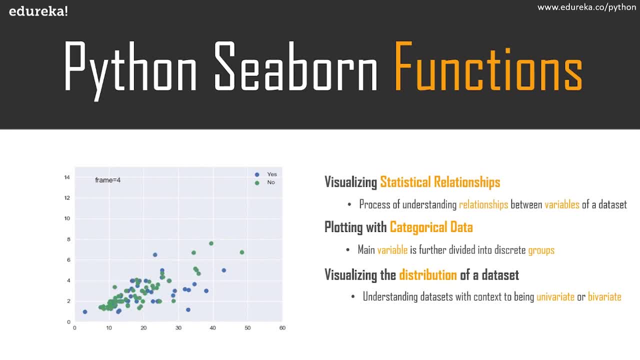 I'll be using the relplot function to plot various statistical relationships. relplot is a figure level function that makes use of two other access functions for visualizing statistical relationships. These access level functions are scatter plot and line plot, which can be specified using the kind parameter of the relplot. 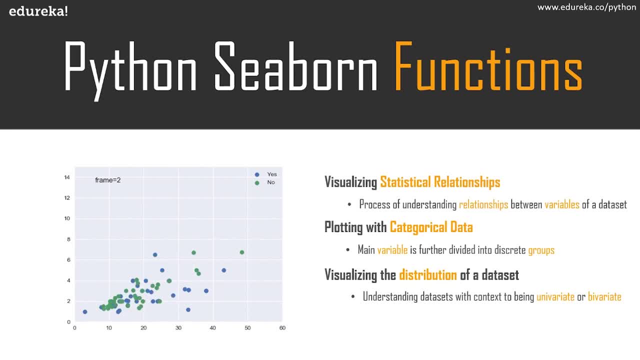 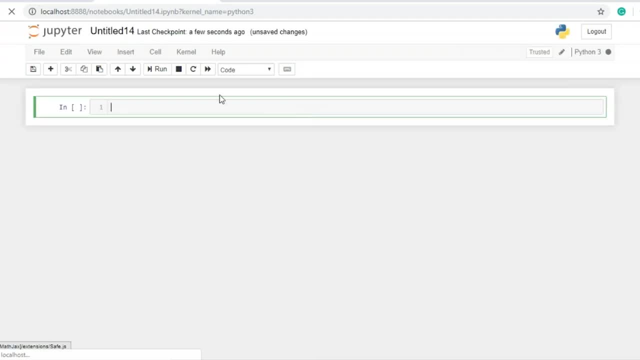 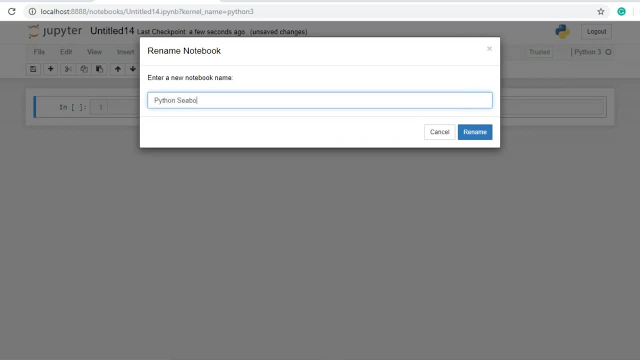 to explain this in detail, Let me jump on to my Jupiter notebook from here. I'll just open a new python notebook. I hope everyone's familiar with Jupiter. Okay, I'll just rename this to python seaborn tutorial. I'll just say python seaborn and I'll rename this. 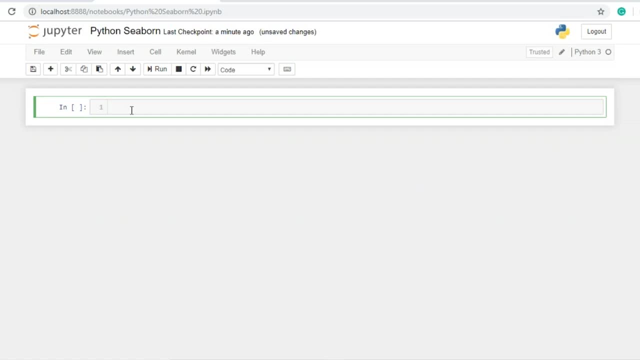 before we begin data visualization with seaborn, We'll have to import seaborn along with its dependencies. So the first thing I'm going to import is numpy: import numpy as NP, Then I'll import pandas as PD, Import matplotlibpyplot as PLT, And then I'll import seaborn, import seaborn. 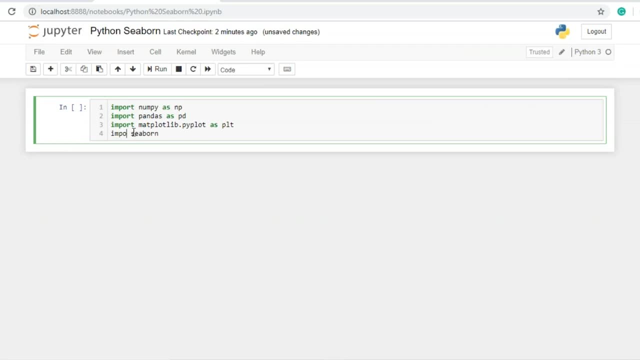 Sorry for the spelling mistake. guys. This is import seaborn, Import seaborn as SNS, and I'll just execute this. like I've already told you all before, you can load any data set present on the github and make use of it with seaborn. seaborn also allows you. 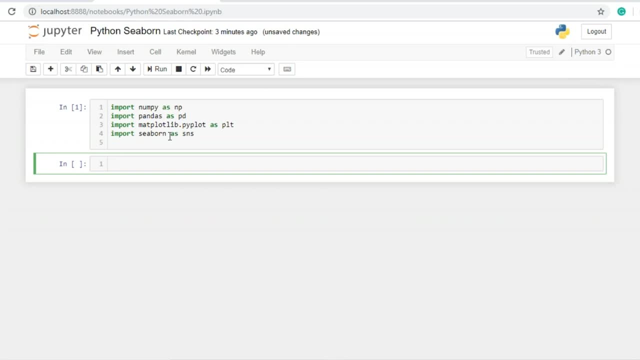 to load any data set from git using the load data set function. So let me just load the flights data set. So I'll just say SNS dot load underscore data set And I'll specify the name, which is flights. Okay, So now let me just go to the github website. 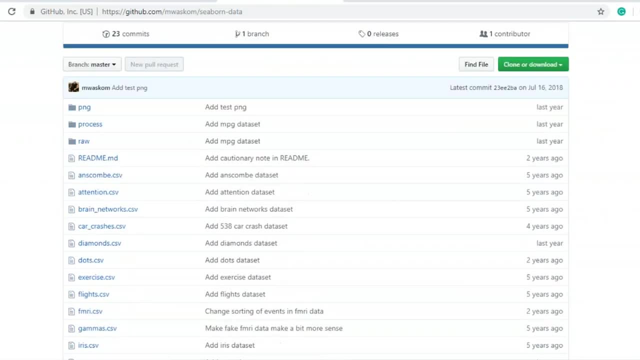 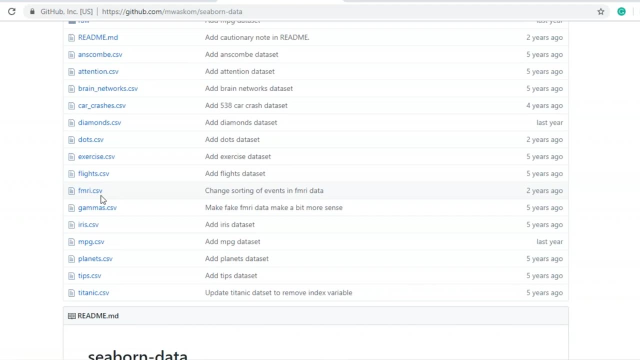 And open the flights data set over here. As you can see, there are a number of data sets that are available which you can use, along with seaborn, So let me just open the flights data set and scroll down. So, as you can see over here, there are three columns. 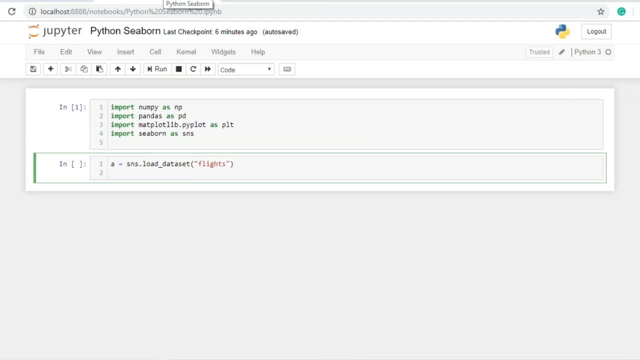 for the year, month and the number of passengers. So I'll just come back to my Jupiter notebook and I'll use SNS dot relplot And I'll specify what I want my x-axis to be. So I'll just give x-axis as the number of passengers. 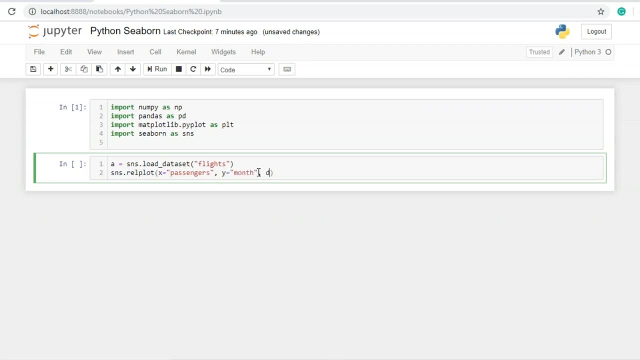 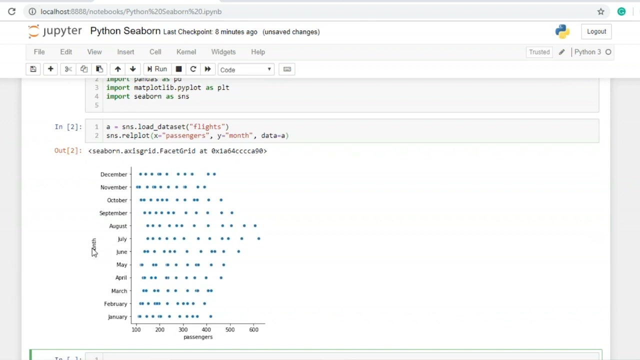 And to the y-axis, I'll give month as the parameter and for the data I'll use a, which is the variable wherein I'm loading the data set, and I'll execute this. Okay, so I hope you're clear with this. So, as you can see over here, the y-axis has month. 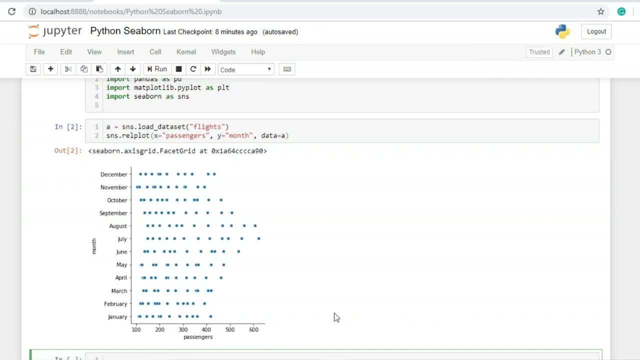 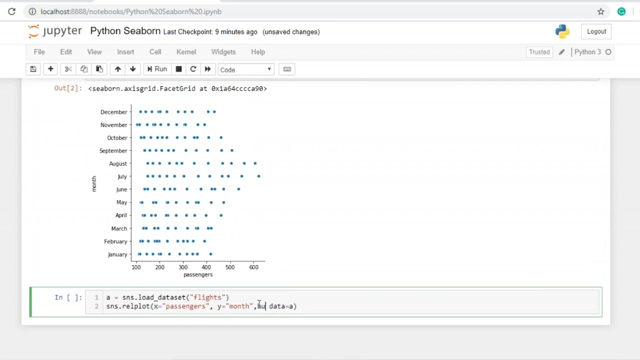 and the x-axis has the number of passengers. These points are plotted in two dimensions. To add another dimension, you can add the hue semantic. So I'll just copy this control C And I'll paste it over here and I'll give another parameter over here. 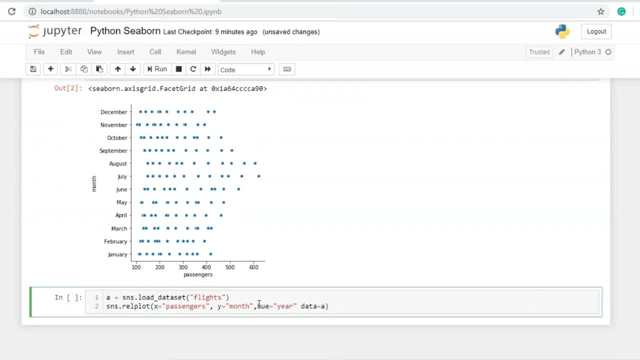 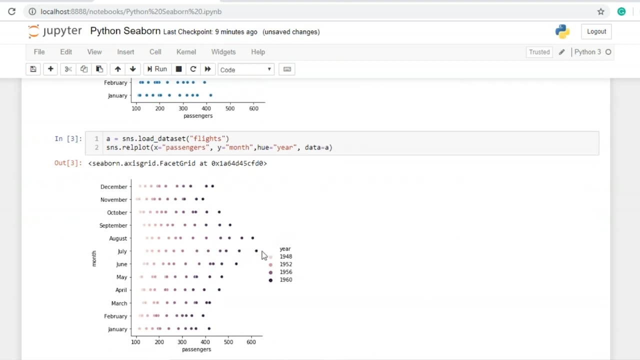 which is hue, and I'll say that is here to be the hue semantic and I'll hit run. So I hope you see the difference. over here The year has been marked as the hue semantic month, which is in the y-axis and the number of passengers. 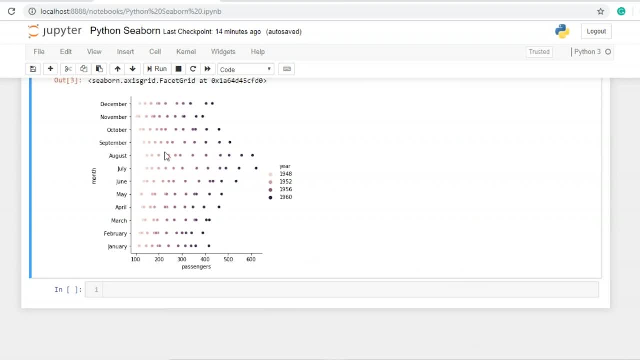 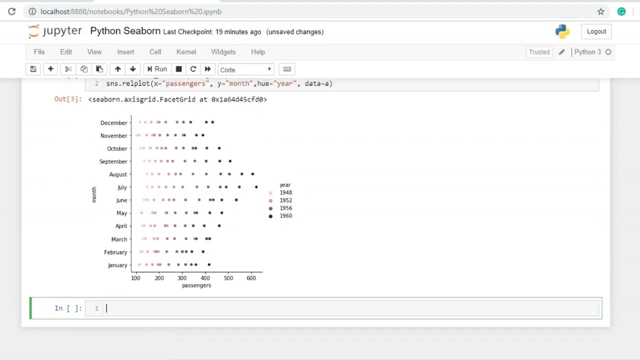 which is on the x-axis. So, as you can see on the screen, this is nothing but the scatter plot. So in case you want a line plot, all you have to do is specify the kind parameter of relplot with the keyword line. 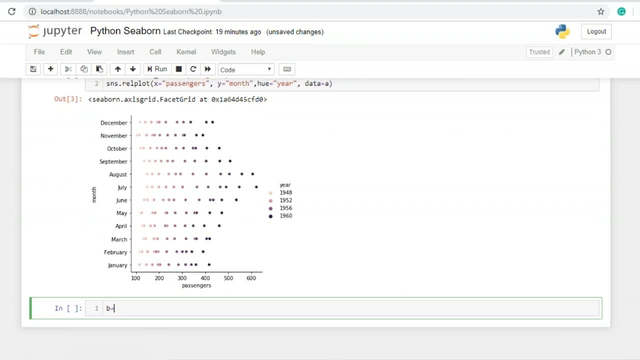 So let me just load another data set over here. So I'll say: B is equal to SNS dot. load Underscore data set and I'll load the tips data set. this time, After this, I'll use SNS dot- relplot. 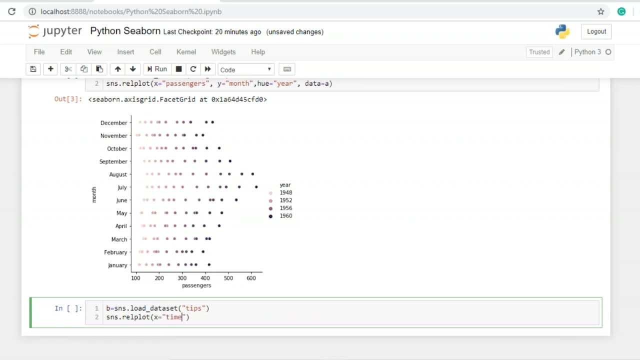 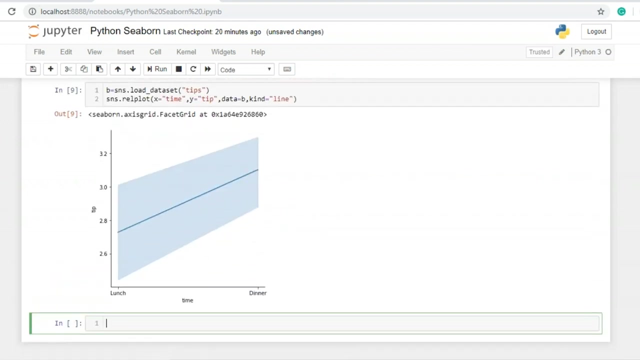 I'll specify the x-axis to be the time And y-axis to be the tip. Data is nothing but B and kind is line. Now let me hit run. Okay, so I hope you're clear with this. If you have any doubts, 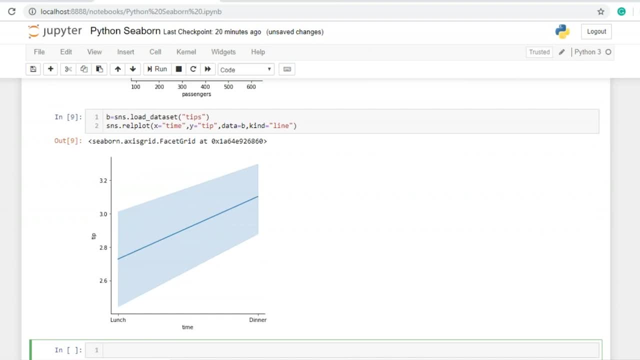 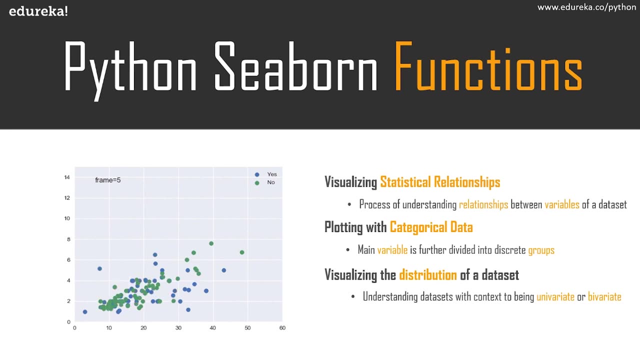 please do let me know in the chat box and my team is here to help you. Now let's get back to our presentation and see how you can plot categorical data in seaborn. This approach basically comes into picture when our main variable is divided into discrete groups. 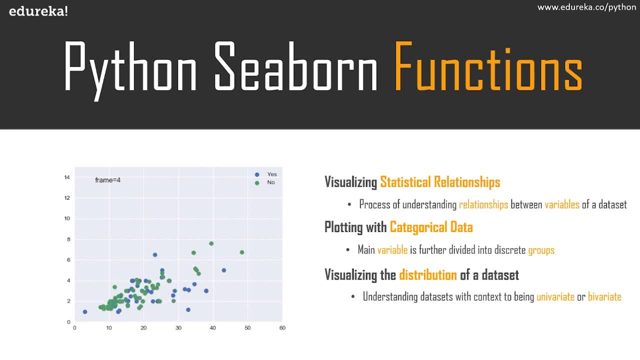 to achieve this, We'll be using the cat plot function available in seaborn. like relplot, cat plot is also a figure level function characterized by three families of access level functions, which are scatter plots, distribution plots or estimate plots. Okay, Now let me jump on to my Jupiter notebook. 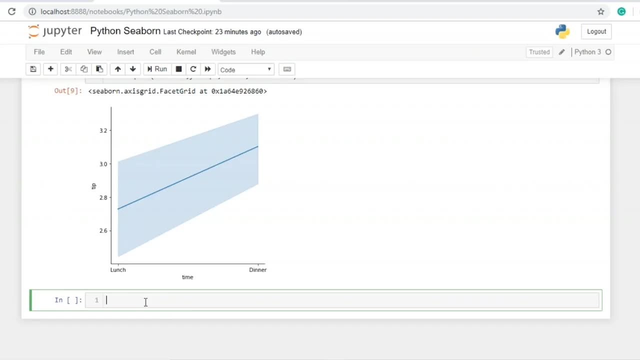 and show you all a few examples regarding this. Okay, So here I'll use the same tips data set and since I've already stored it in the variable B, I'll just use SNS dot cat plot And I'll specify the x-axis to be the day. 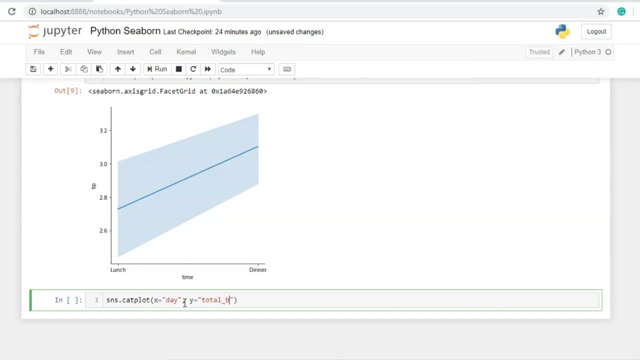 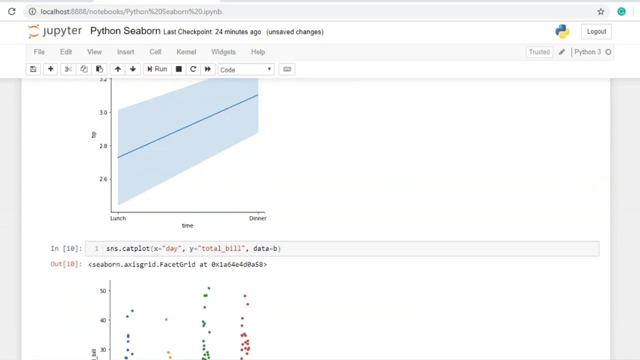 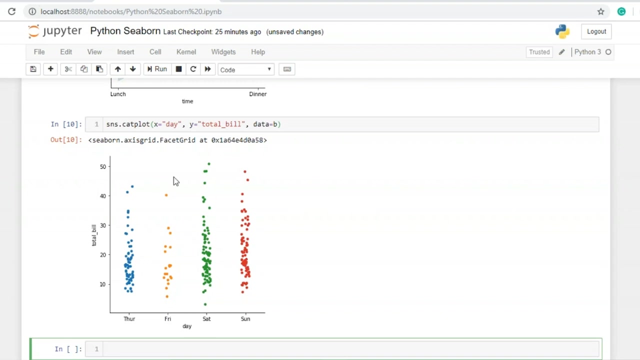 Y-axis as the total bill And data is B. Now let me hit run. Okay, as you can see over here, This is the scatter plot that we've got using the cat plot function. Scatter plot is basically the default type of cat plot. 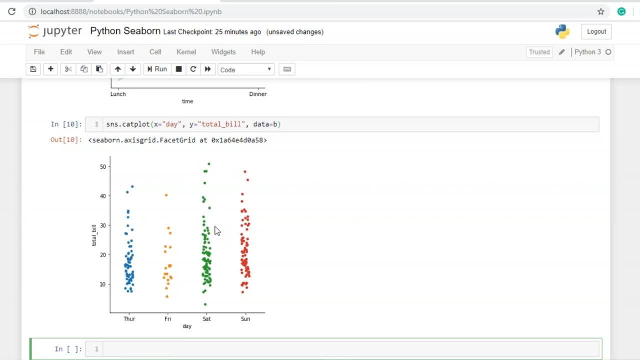 However, you can change the kind of plot you want by specifying the kind parameter, like we've done previously. You can choose between any options, which is strip plot, swarm plot, box plot, violent plot, Etc. Let me just show you what happens when I change the kind parameter of this cat plot. 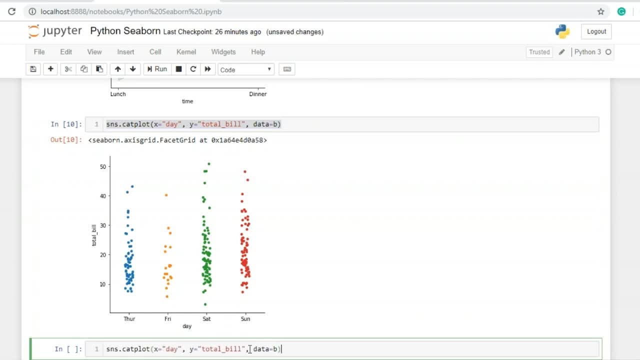 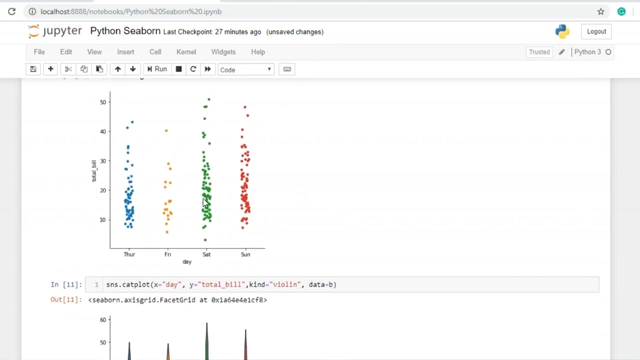 So I'll just copy this and I'll paste it over here and I'll specify kind to be as violent plot. So I'll specify the keyword violin and I'll hit run. Okay, so I hope you see the difference. This is our scatter plot and this is our violin plot. 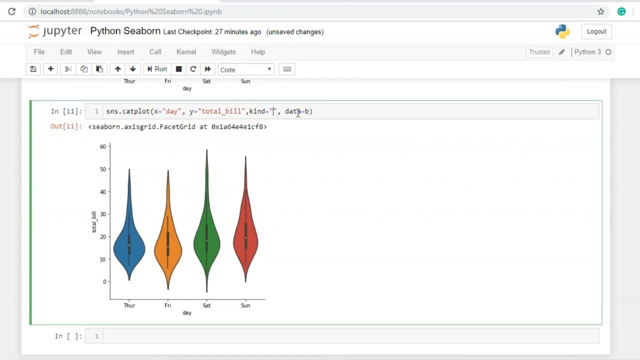 So if I change the kind parameter, our plot will change correspondingly. Let me just give the type as box in now. Okay, so I hope you're seeing the difference, guys. So now let's get back to our presentation and see how to visualize the distribution of a data set. 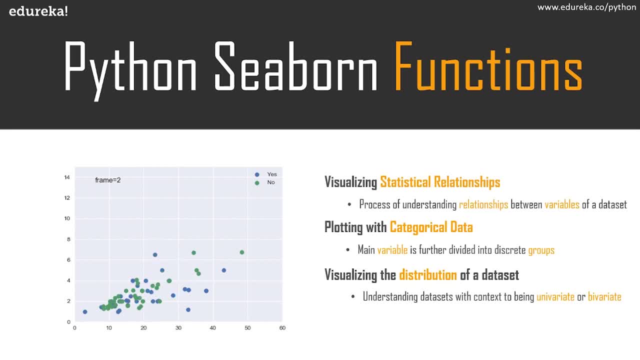 visualizing data set basically deals with understanding data sets with context to being univariate or bivariate. Okay, So now let's get back to our Jupiter notebook and see how you can actually plot univariate and bivariate distributions. So before doing this, 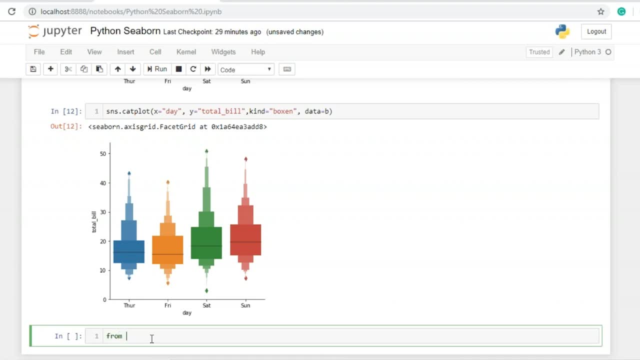 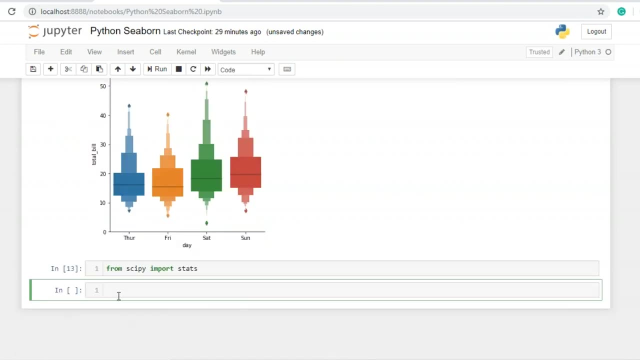 I'll just import stats from the scipy library. So from scipy, import stats and I'll hit run. Okay, So first let us plot univariate distributions. to plot univariate distributions You can use the dist plot function. So let me just take an example. C is equal to NP. dot random. 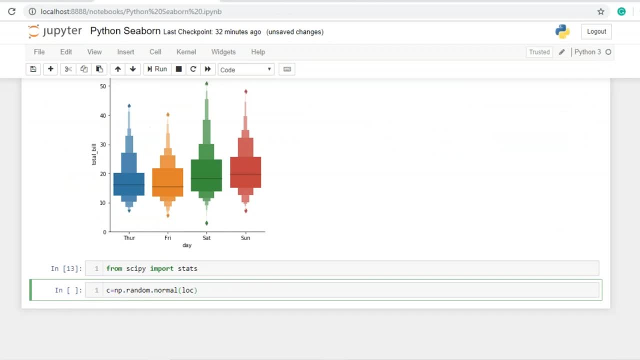 I'll just use random, Not normal functions to draw random samples from a normal distribution. So I'll just give the corresponding parameters to it. You can give any parameters of your choice, Let's say size equal to 100 and scale. I'll specify the scale to be as do, and I'll hit run. 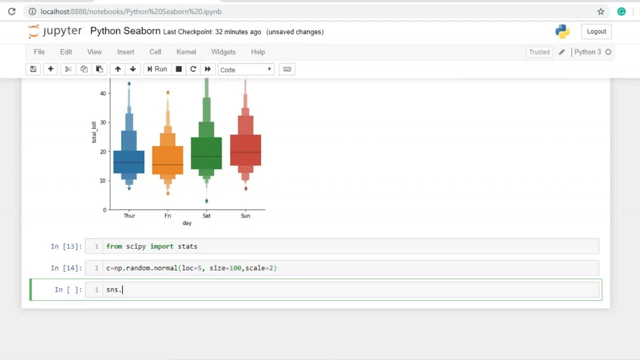 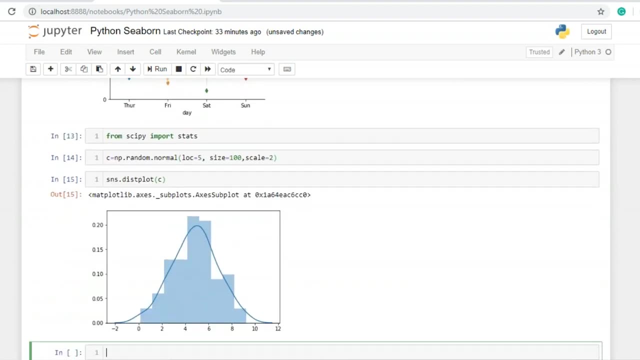 I did not specify the dist plot function, So I'll use SNS dot dist plot and I'll pass the data to it as see. Okay, So this is how the dist plot function works. So this is an example of a univariate distribution. 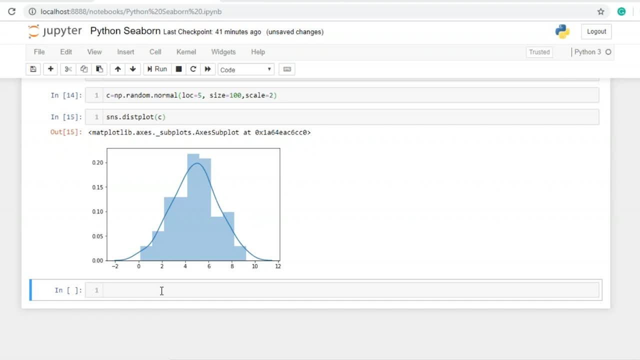 So now let's move on and see how a bivariate graph is going to look. To plot bivariate distributions, You can make use of the joint plot function. I already have a small example typed over here, So I'll just copy paste that. 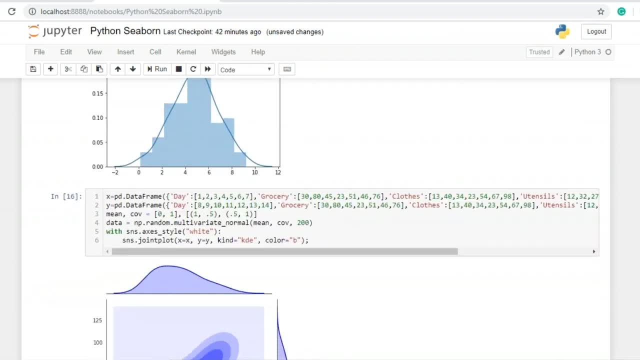 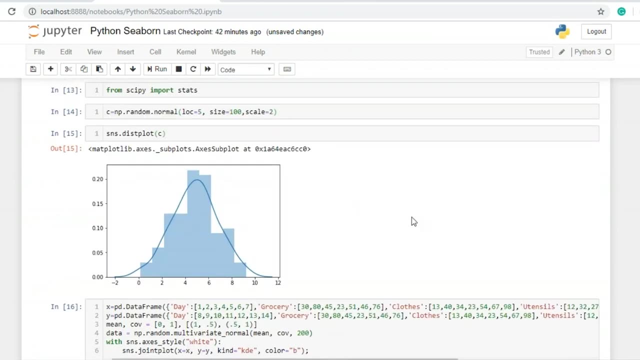 and I'll show you all how it actually looks. Okay, So this is basically a bivariate distribution. So I hope you see the difference. This was our univariate distribution and this is our bivariate distribution. Okay, if you have any doubts. 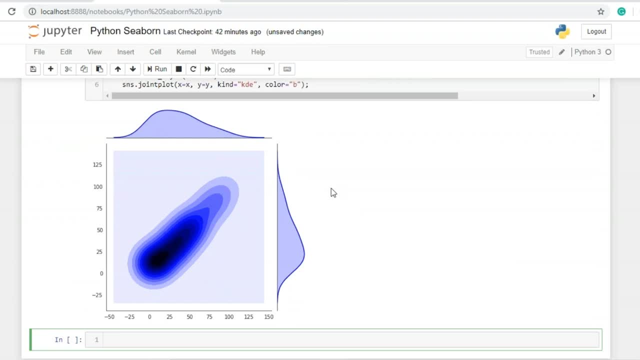 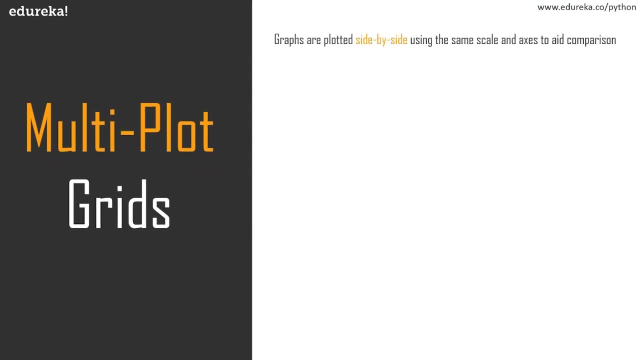 please do let me know in the chat box and my team is here to help you. Moving on, Python cvon also allows you to plot multiple grids side by side. These are basically plots or graphs that are plotted using the same scale and access to eight comparison between them. 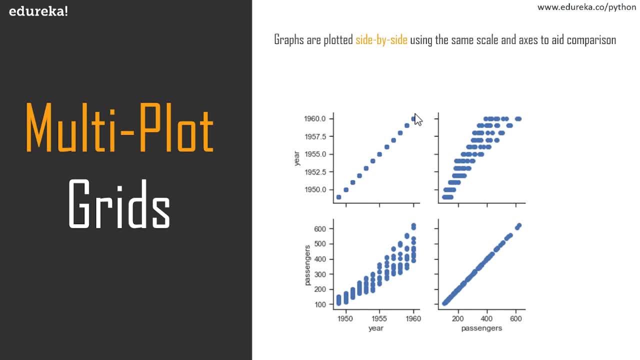 This in turn helps the programmer to differentiate between the plots and obtain large amounts of information. to plot multiple graphs, You can either use the facet grid function or the pair grid function of cvon. Let me jump on to my jupyter notebook and show you all an example of each of these. 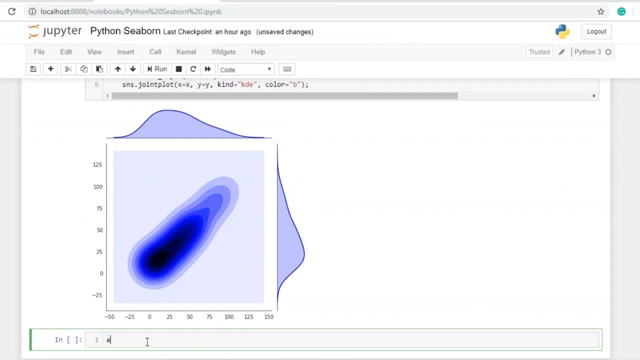 So first I'll be using the facet plot function, Okay. So here I load another data set, So I'll just say a is equal to SNS. dot load data set. And this time I load the iris data set And I'll say B is equal to. 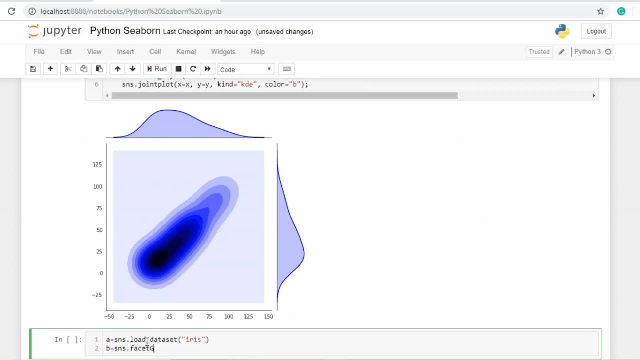 SNS dot facet grid, which is the name of our function, And I'll specify a where and where in our data is present and I'll specify the column to be the species. I'll specify the column as a species of flowers and then I'll just use the map function. 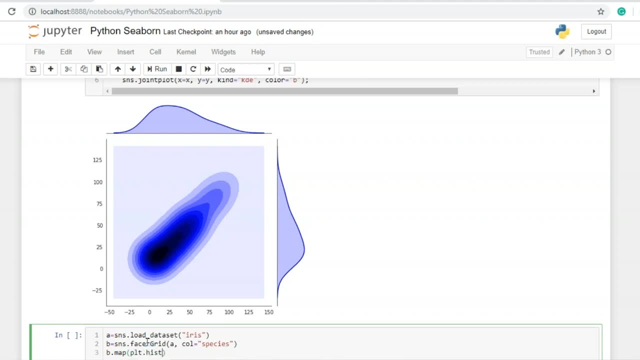 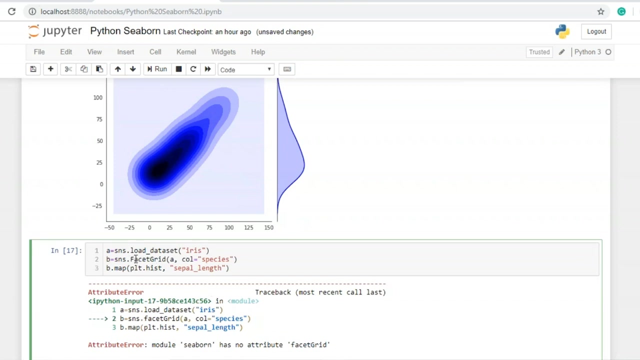 And I'll specify all of them to be as histograms And I'll give the parameter as sepal length. Now let me hit run. Oh sorry, I made a spelling mistake of here It's capital F. Okay, So I hope you're clear with this. 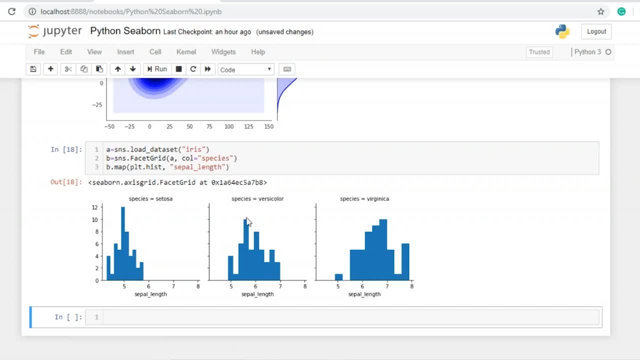 I basically have three graphs that are available for the three species of flowers, which is setosa, versicolor and virginica. As you all can see, it becomes very easy to differentiate between them. You can also make use of the pair grid function when you have a pair of variables to compare. 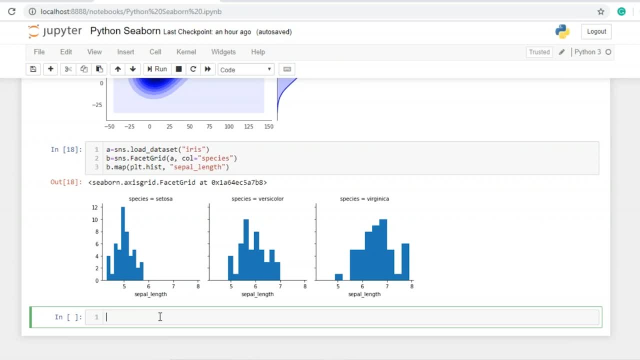 Let me show you a small example of that as well. So here I'll just say: a is equal to load underscore data set And I load the flights data set And then I'll specify B as SNS dot pair plot Bear grid. sorry. 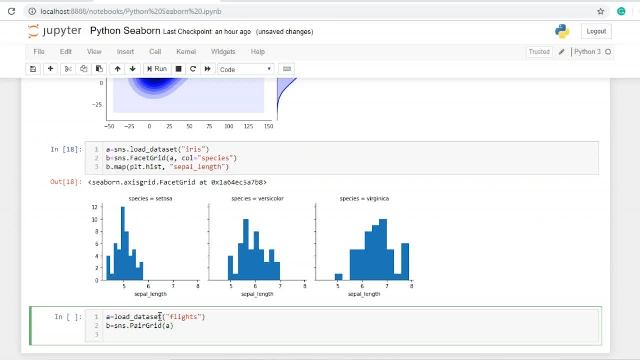 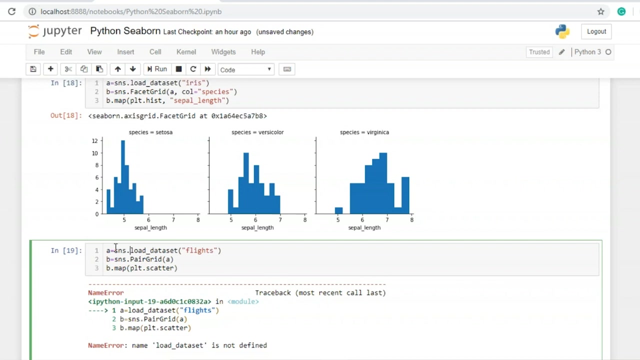 And I'll specify the data to this as a and I'll use the map function again to plot them. this time I'll use scatter plot, So PLT dot scatter. Sorry guys, I forgot to specify SNS over here. SNS dot load underscore data set. 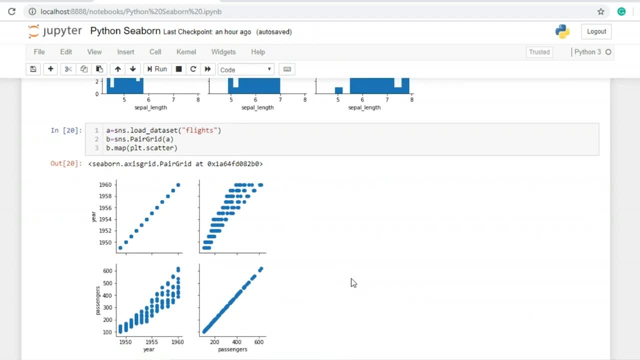 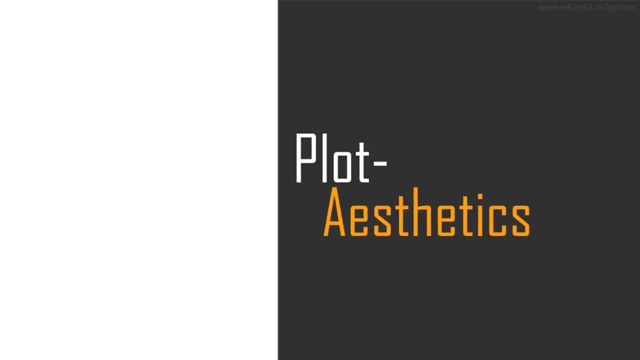 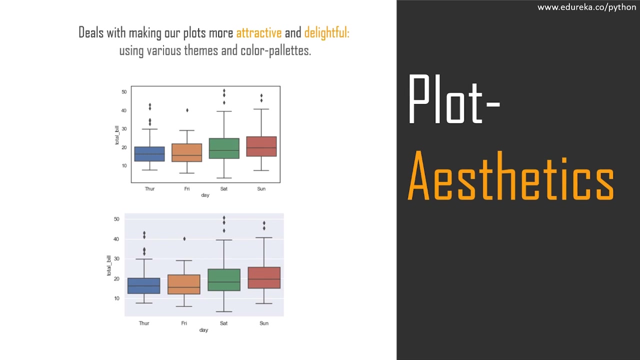 Okay, so I hope you're clear with this. So, as you can see, the output clearly compares between the year and the number of passengers. In different ways, Seabourn also allows you to make your plots more attractive and delightful. So till now, as you've been seeing, I've just had a white background. 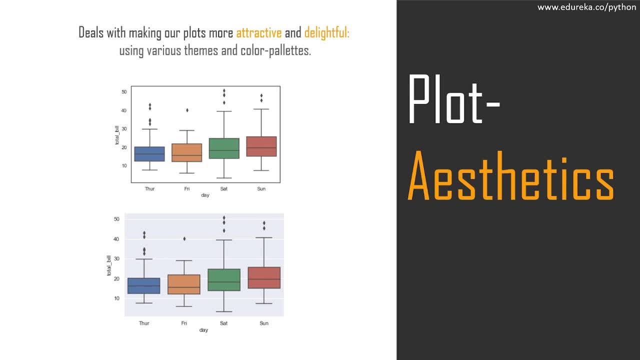 for all my plots. So in case I want to change this, or if I want to change the color palettes that are available in my graph, I can do so easily. Let me just jump on to my Jupiter notebook to show you all how to do this. 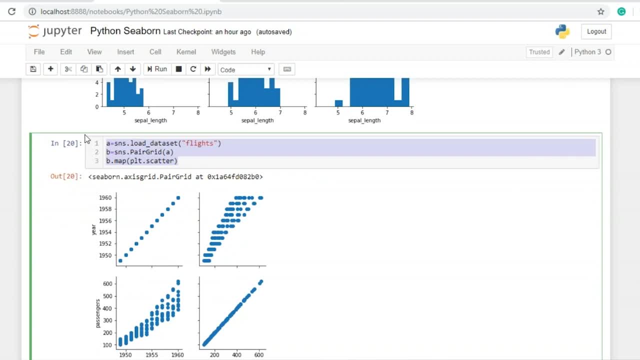 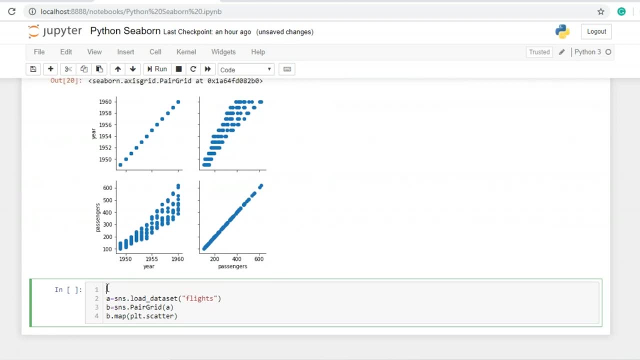 So here I'll just copy paste the previous example, I'll just copy this And I'll paste it up here. And to this I'll just use another function, Which is the set function, And I'll specify the style, the style of my plot. 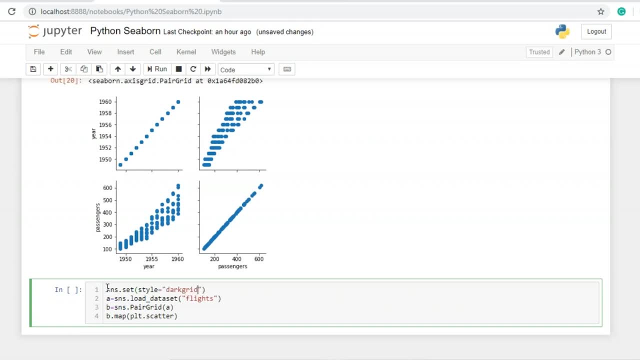 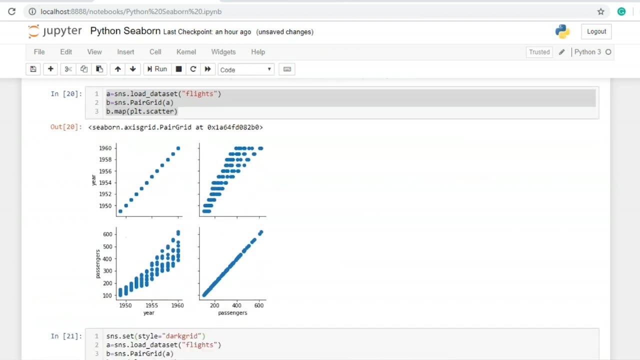 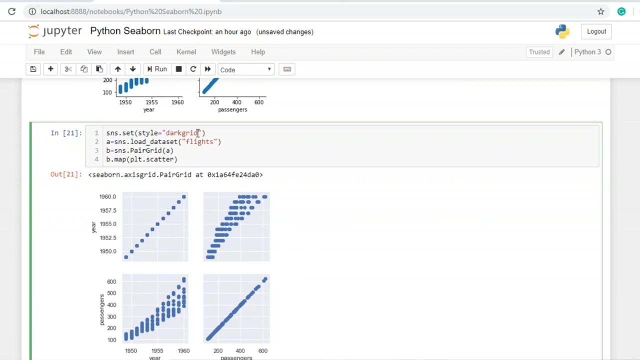 to be dark grid And I'll hit run. I hope you see the difference between the two. here I have a white background, Whereas when I specified dark grid, I have a different background, with dark grids that are seen clearly. you can change the style parameter. 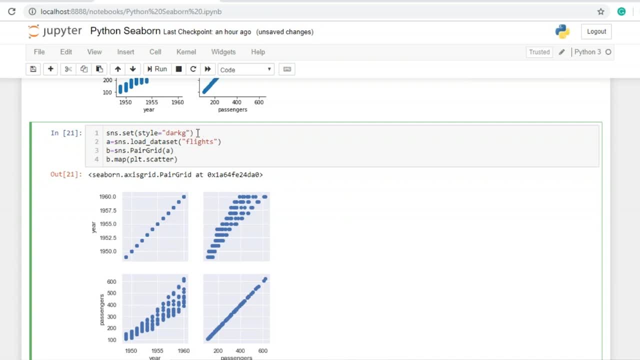 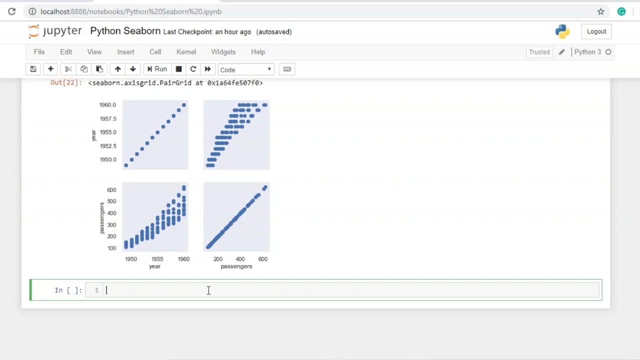 to any of the available Themes, which is dark grid, dark white, Etc. So if I just specify dark and I hit run, you can see that the grids have vanished, but the background is dark, Not just this. guys, you can make many of the changes to your graphs. 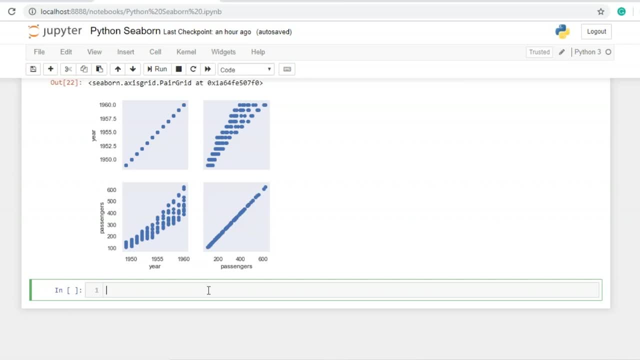 such as adding or removing access, the colors that are available, Etc. Now let me just show you all how you can remove the axis lines that are present in your graphs. I'll take another example of yours, or SNS dot set. I'll set the background this time as white. 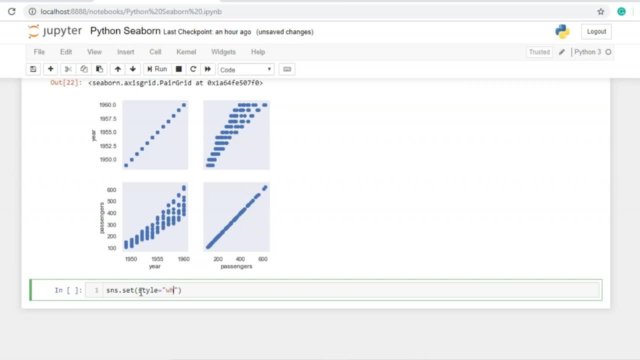 I'll say style Equal to white And I'll specify the color Color code parameter to be true. I load the tips data set again. SNS dot load data set and I load the tips data set. Then I'll use a box and plot. 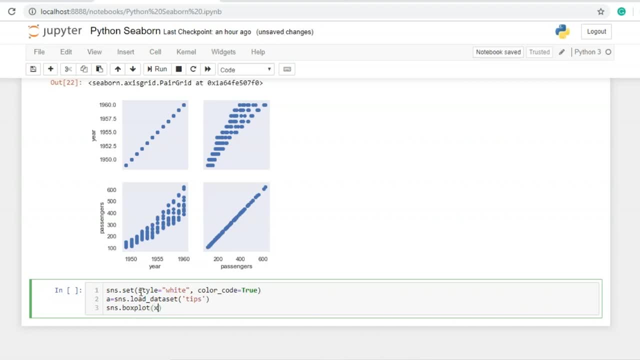 Or I've used the box and plot. So this time I'll use the box plot function and I'll specify x-axis to be the days- and sorry, it's day, not days- and the y-axis to be the total bill. And data is nothing but a oh, sorry guys. 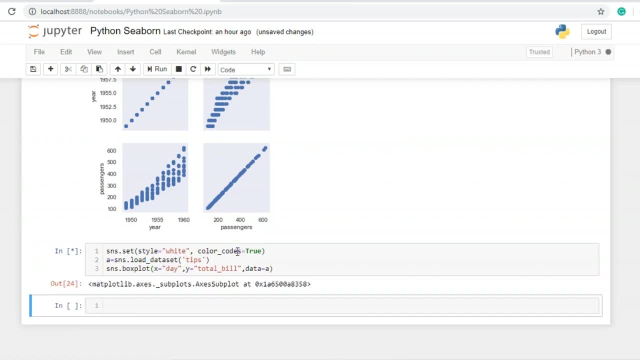 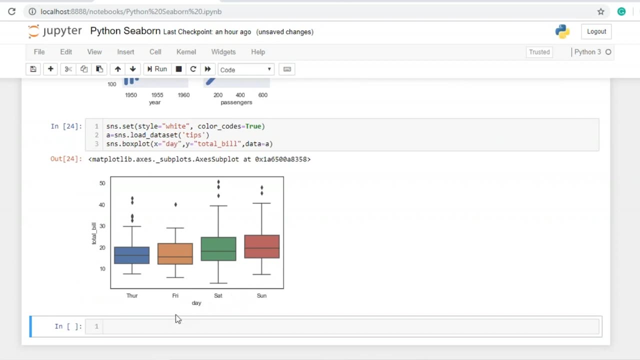 I've made a spelling mistake Of your color codes. Okay, So here, as you can see, my plot has access all around it. nice, I want to remove any of these access. All I can do is use the despine function, So I'll just copy paste this.